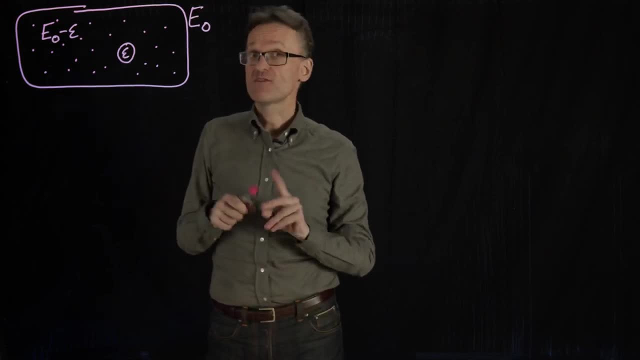 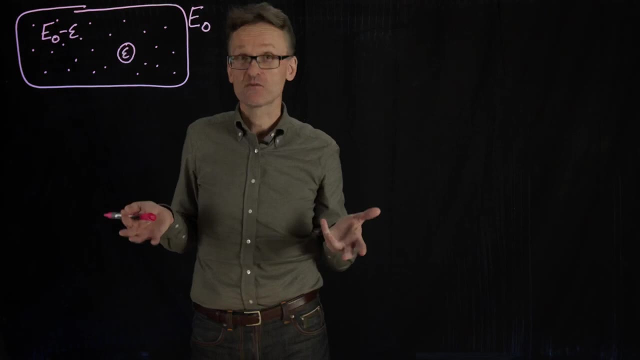 And I already hinted and it's going to make it very clear now that the likelihood of observing a system in a particular state- well, that's simple. It's just proportional to the number of ways I can find the system in that state. Compare that to the previous slide in orange. right, If it's a well. 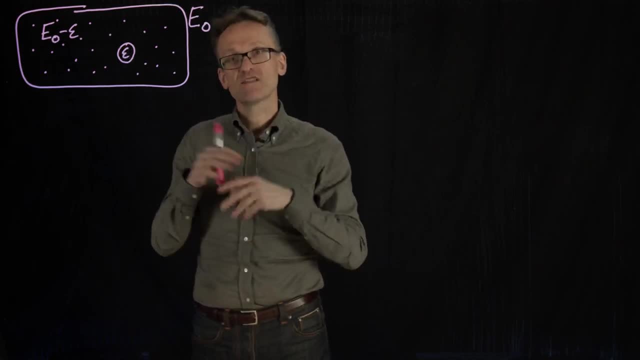 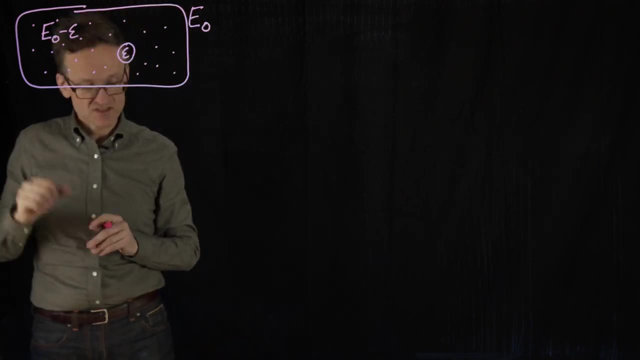 ordered system. there are a few ways we can put it that way, while there are many disordered ways. So this, and this is the first part- I'm going to need to define something And I said that I'm interested in the probability of observing a system. 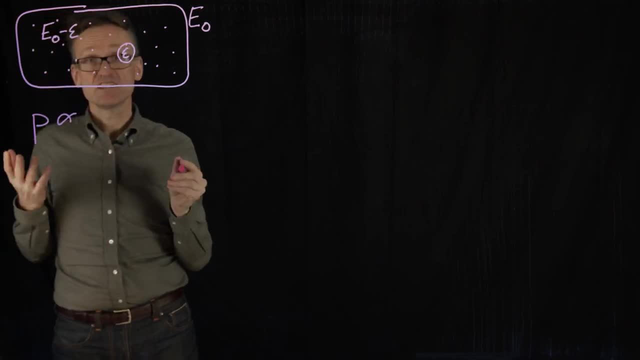 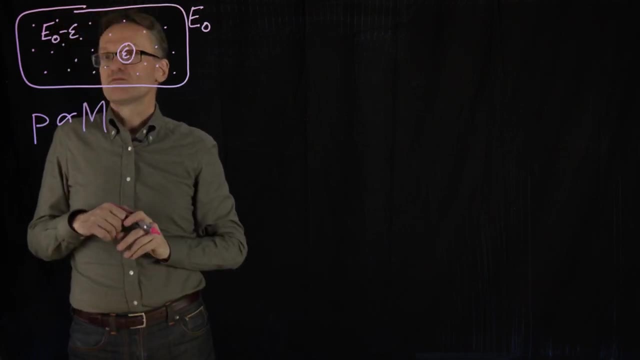 And that probability p is proportional to the number of states. I'm going to need to call that something. I will follow the book and call that m. We typically call this a thermostat or something, but that's the only system I'm going to be. 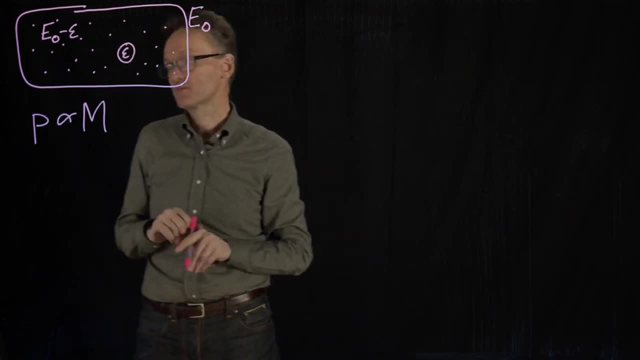 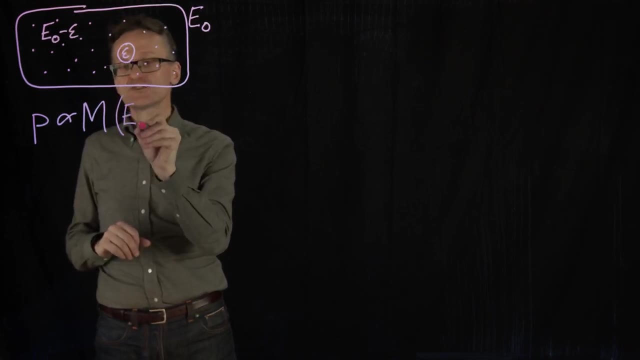 considering. so I will skip the suffix here to save some space on the board. But the number of states here in general is a function of the energy, And the energy for the rest of the system here is E0 minus epsilon. Because, again, 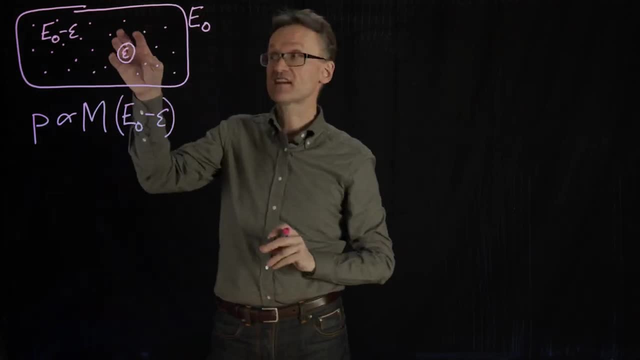 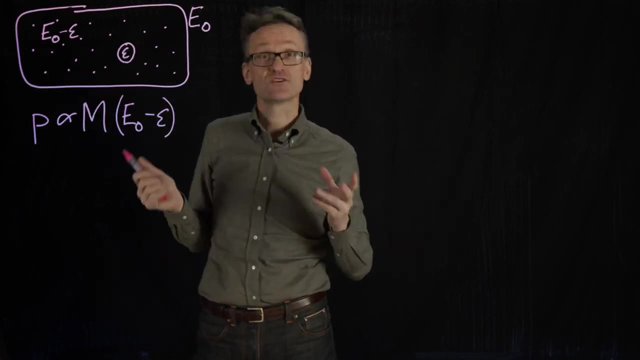 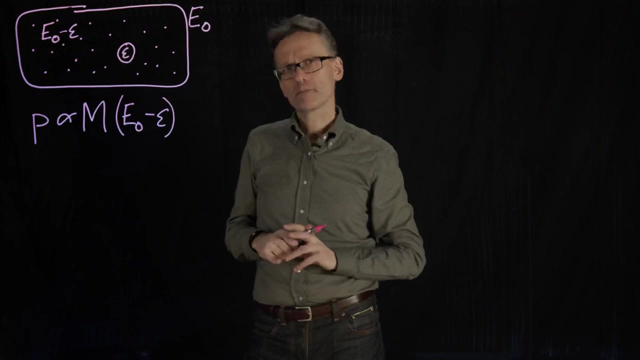 this is the small part of the system that I'm not considering. That is one that is well defined, That is a specific state right. It's these other states that I'm allowed to distribute and consider how many of them I have. I don't know anything more about that, literally, Or do I? Well, I know. 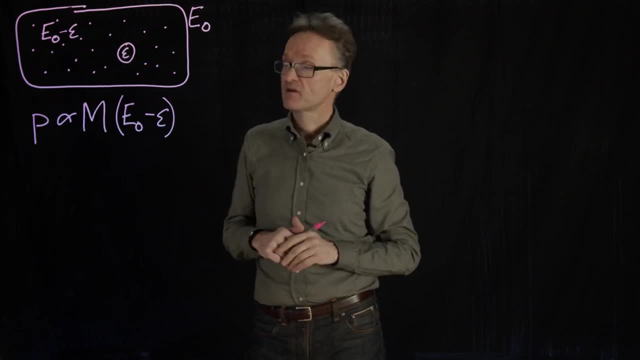 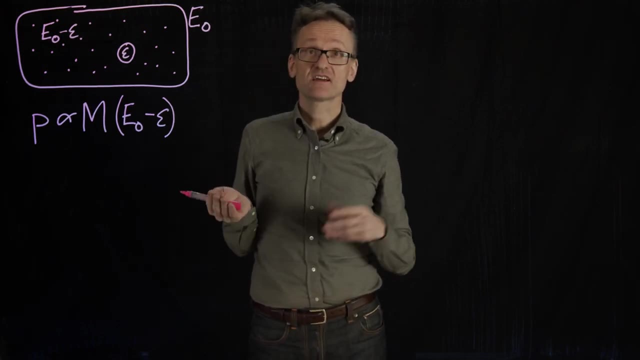 that it's a positive number, because there should be at least one state. The other thing with probability is that they're a bit of a pain to work with. If I have one coin here that's head or tails and one coin here that's head or tails, They have two possibilities each, but 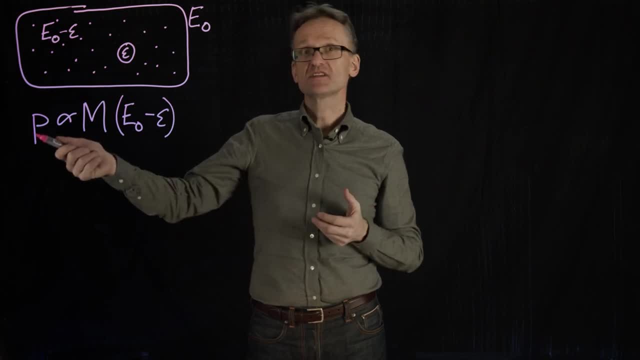 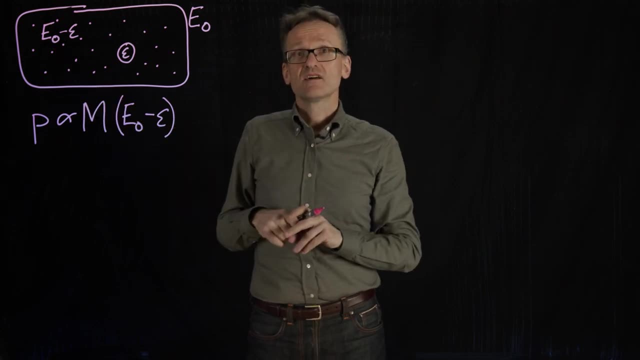 if I start grouping coins and I talk about probabilities, that means I should multiply probabilities. That's a bit awkward because when I talk about energies we're used to summing them. There is a very easy way to get the same property here. I will just introduce another. 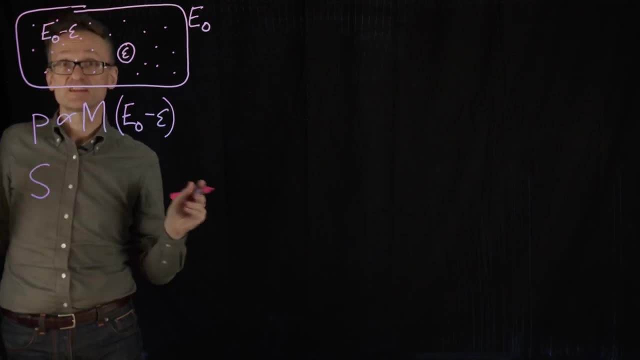 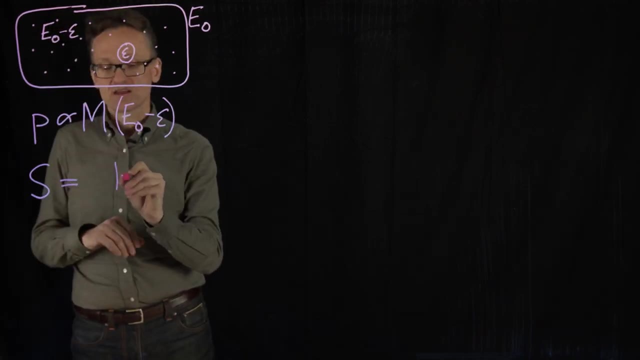 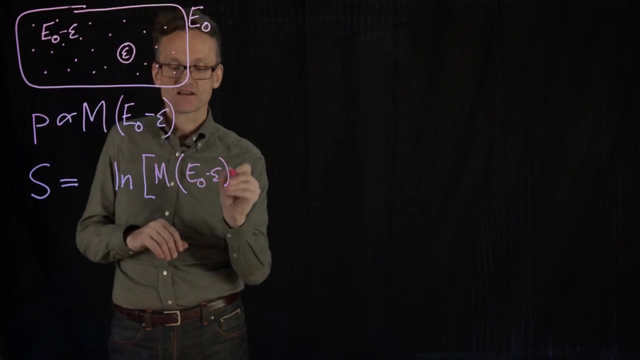 number, or whatever we call it here: S, Don't think about this. S I could have used Z if I wanted to. S is the number of the state. S equals- leave some space. logarithm of the number m of E, zero minus epsilon, And then I might want to have some units here or so. 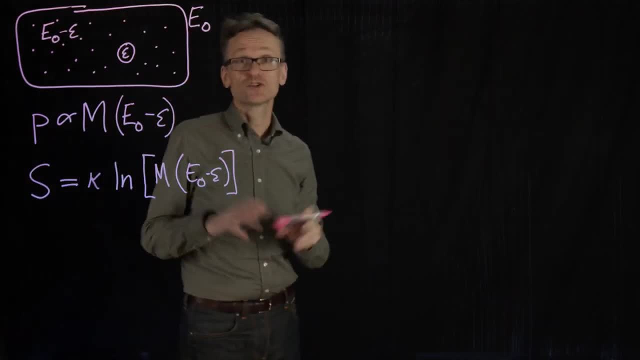 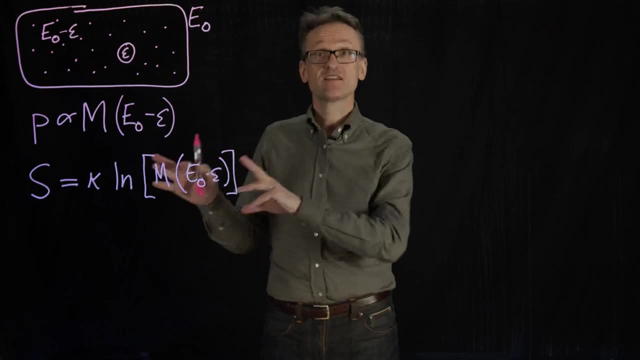 so I'll just say that there is a small unit that I will call kappa, just a constant. I'm always allowed to take the logarithm of something that's neither zero nor negative, so that I haven't simplified or assumed anything. It's just a pure mathematical definition. But now, if I 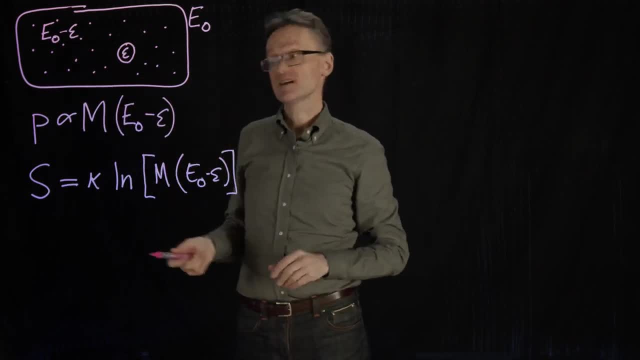 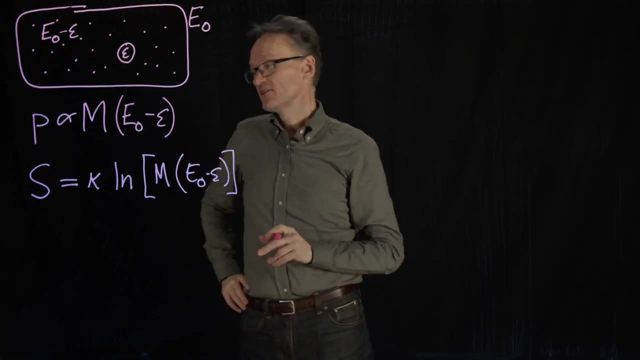 double. if I take two systems like this, I should double the energy and I should double S, So that makes them easy and behave in similar ways. But I still don't know. I didn't know much about m. I don't know a whole lot more about S. 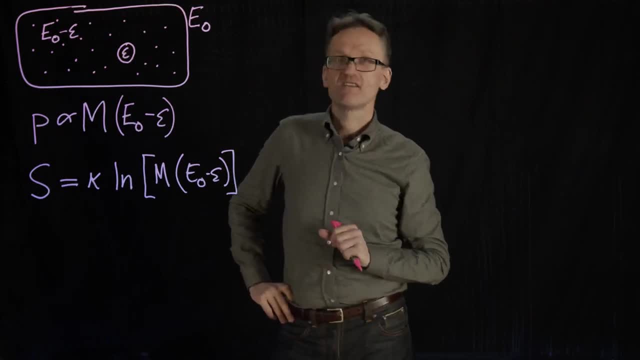 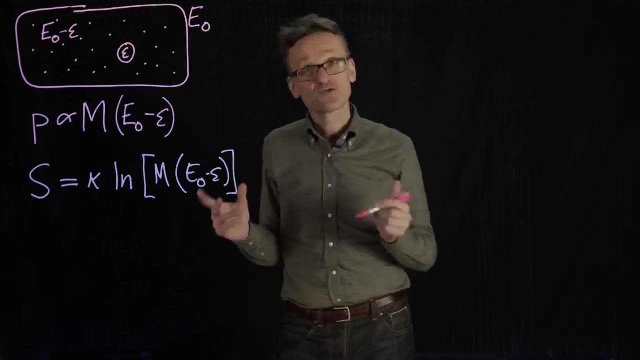 Remember when we defined bonds and what a physicist did when there was some complicated function I didn't really know the shape of. I made a series expansion around something that I knew. Let's try that here. So let's do a series expansion of S. 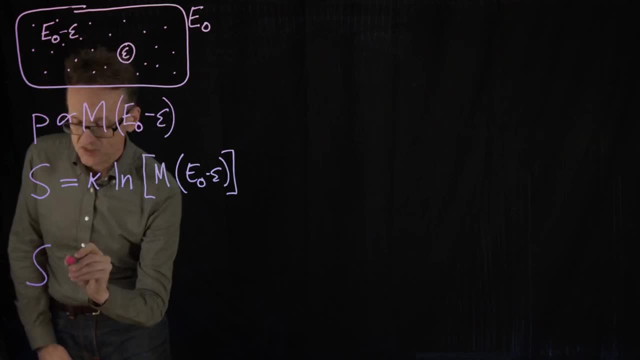 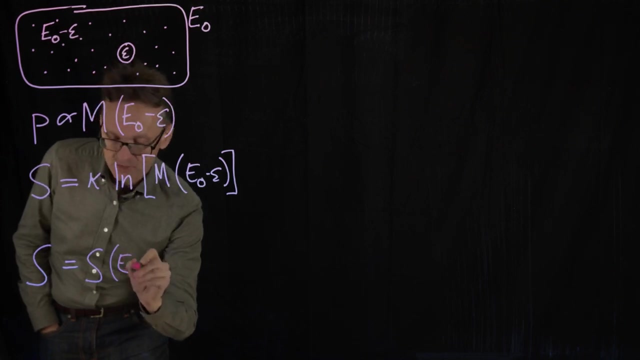 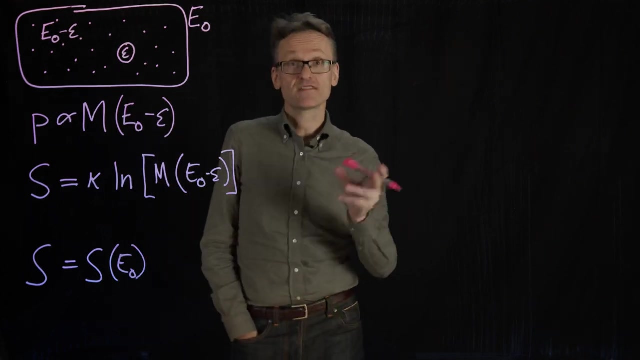 and say that S is approximately equal to, but I'm going to write equal for now, So let's expand this around the value E zero. So S is then equals S at the value E zero, plus the displacement from that value multiplied by the derivative right. That's the first order. 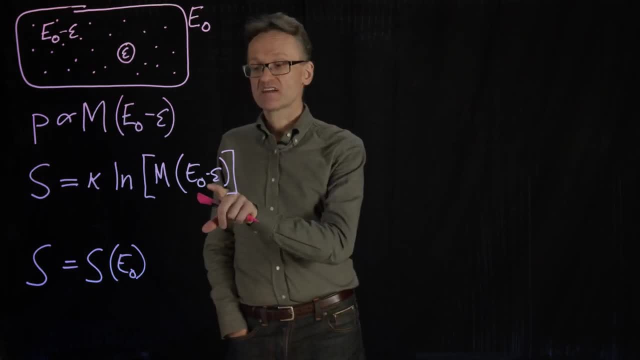 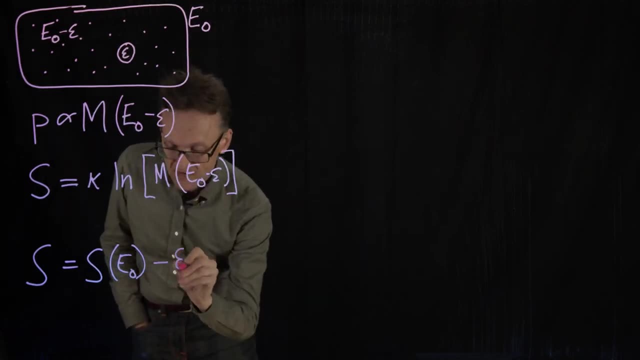 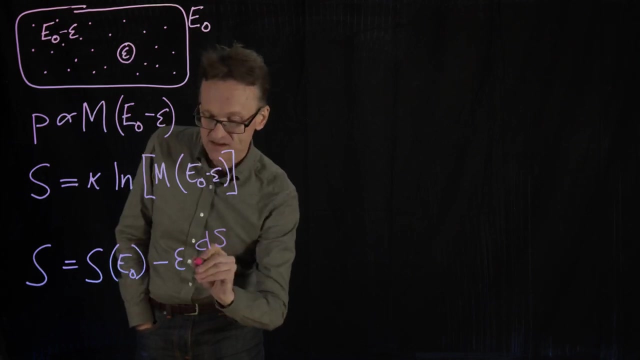 component. But the displacement I'm going to looking at is what I'm adding here, and I'm going not adding, I'm actually subtracting. So it's going to be minus epsilon. So it's minus epsilon multiplied by the derivative of S, which is a function of E with respect to energy taken at. 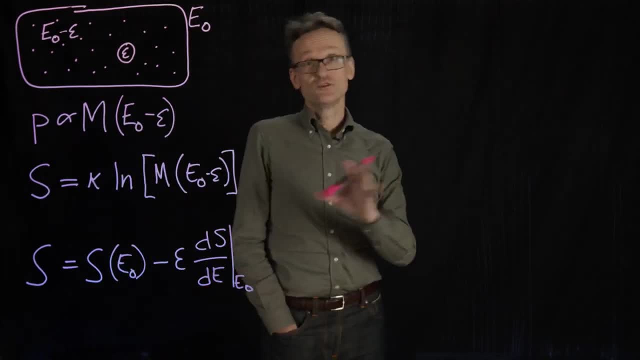 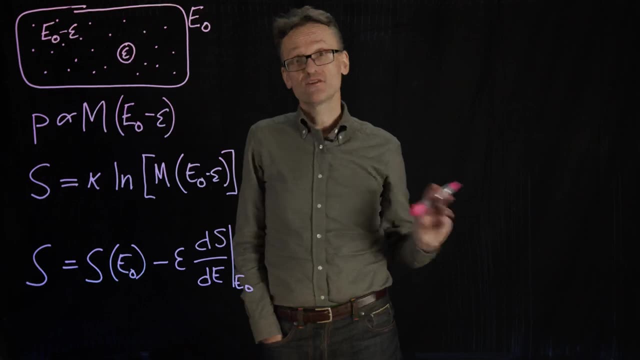 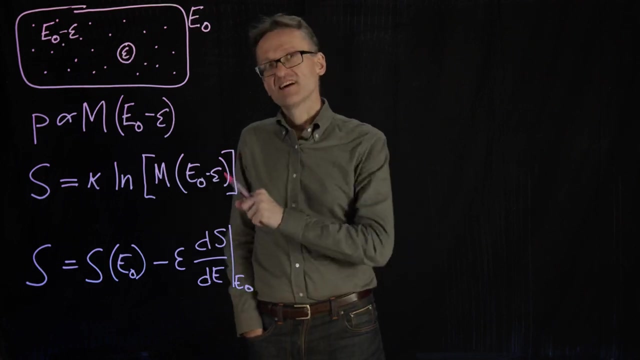 the value E zero. Just first order expansion, Taylor expansion, And now I'm going to need to continue this with a second and third and fourth order term. Or should I just make do here and say that we're good enough? Yes, And here we're going to use a trick. Remember that I said that S was. 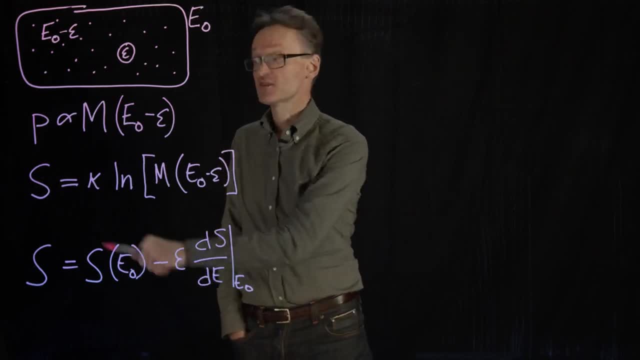 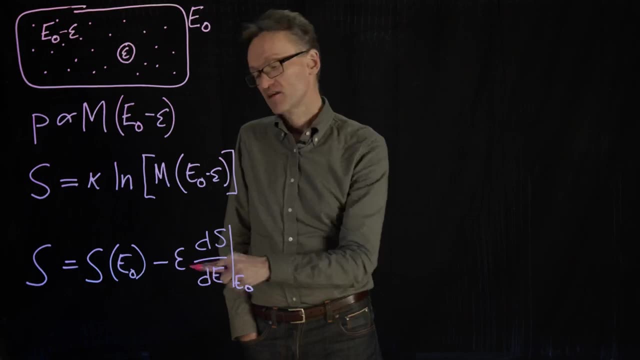 proportional to the size of the system. If I double the size of the system, I will double S. That means that that term will go up as the size of the system. So I definitely need that one Here. epsilon is small, but here I have a quotient of something in the nominator that is proportional. 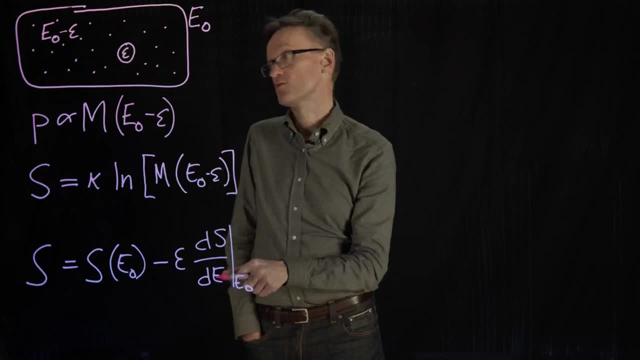 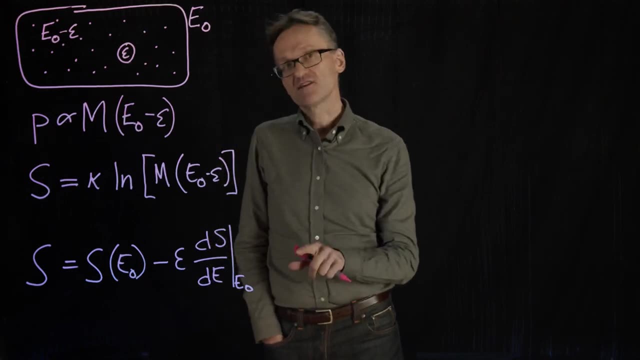 to the size of the system and something in the denominator that's also proportional to the size of the system. So I'm going to say that we're good enough. Yes, And here we're going to use a trick: That's going to be a constant term. I need that, But if I were to take a second derivative here, 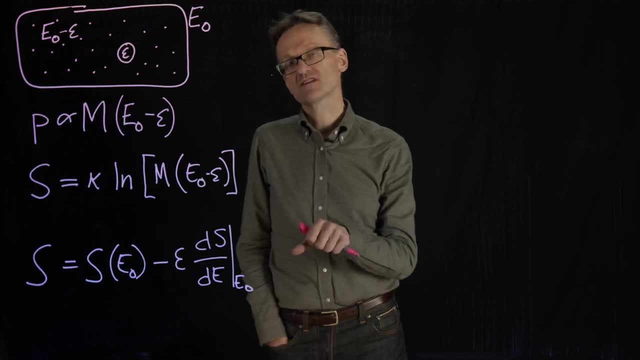 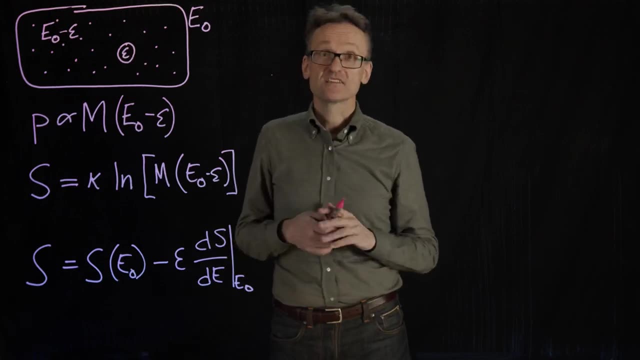 I would have something in the nominator that is proportional to the size of the system divided by the square of the size of the system. And the trick with statistical mechanics is that we study very large systems: ballpark of 10 to the power of 23 atoms, right. 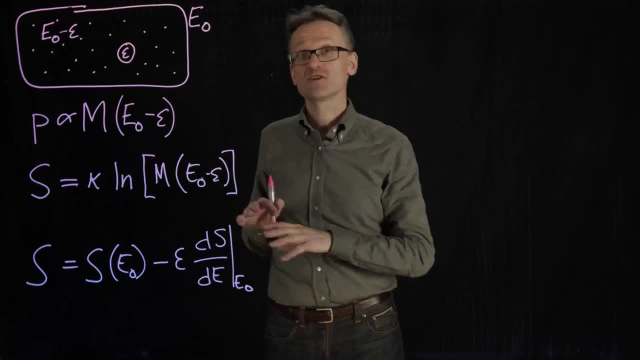 If you divide one, divided by 10, to the power of 23,, it's going to be so large that we can literally ignore anything beyond this first order term, And this is going to be a constant term. But if I were to take a second derivative here, I would have: something in the denominator that is proportional to the size of the system. divided by 10, to the power of 23.. So if I were to take a second derivative here, I would have something in the denominator that is proportional to the size of the system. and that's going to be so large that we can literally ignore anything beyond this first order term. And this is going to be so large that we can literally ignore anything beyond this first order term. So it's not really a simplification for a system that's large enough. 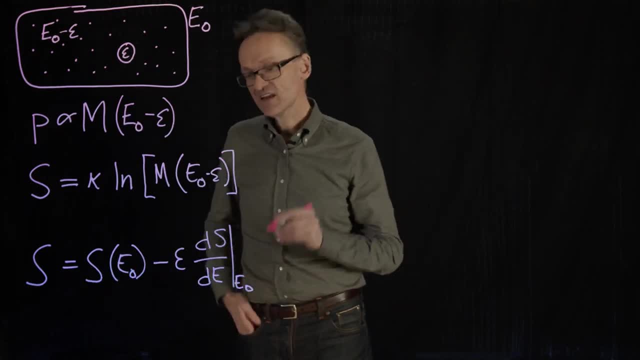 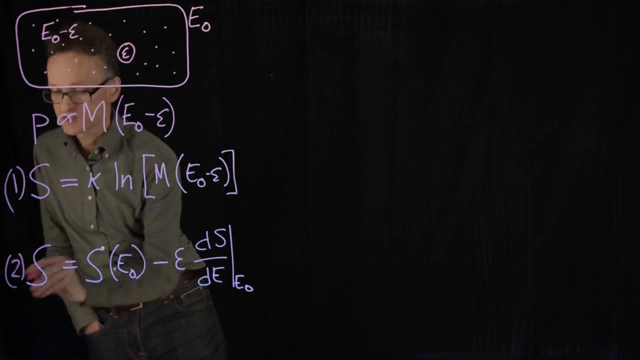 So now I have a much simpler expression for this. Let me call these something that. let's say that the first one here was equation one And the second one was equation two. I'm now going to solve for m, because I really wanted m, right. 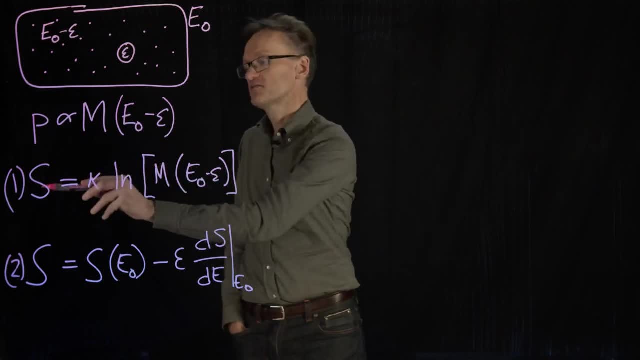 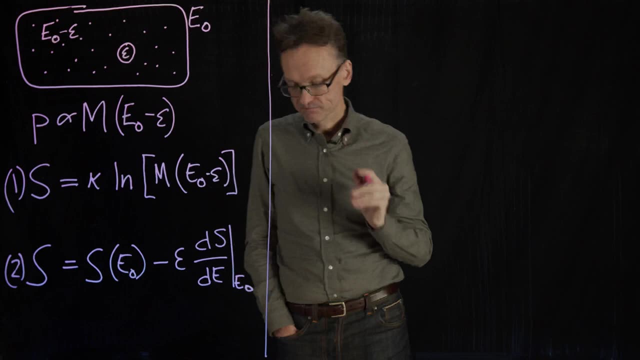 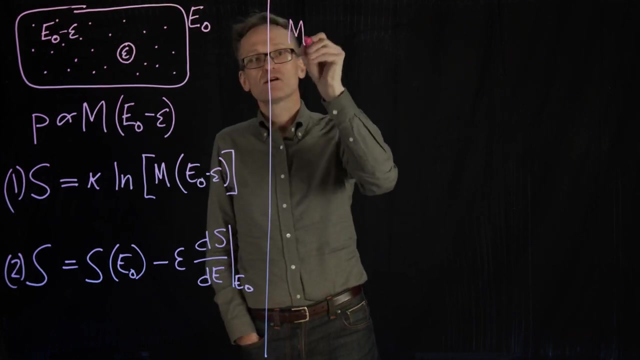 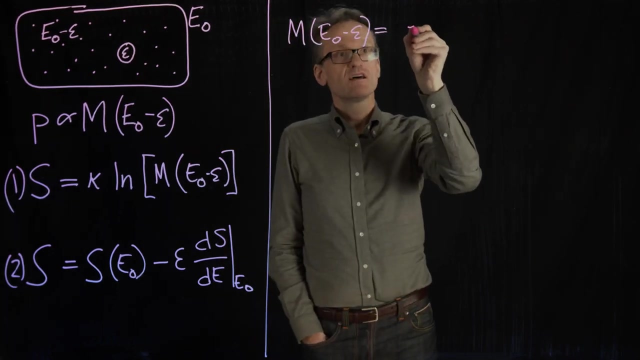 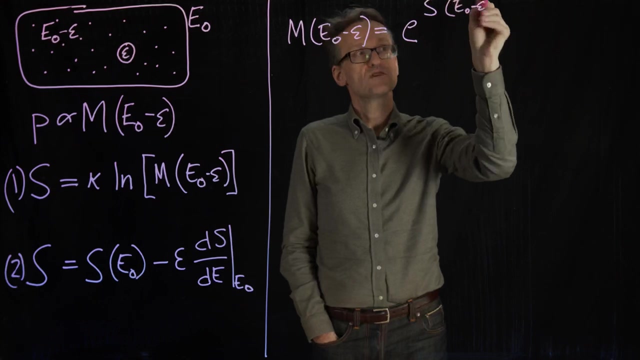 I'm going to solve for m in equation one, But instead of saying s, I can use equation two. So where will that lead us? Well, This is easy. I will take s divided by kappa, and then take the exponential, So that m of e0 minus epsilon is equal to e raised to s, which again is a function, then, of e0 minus epsilon divided by kappa. 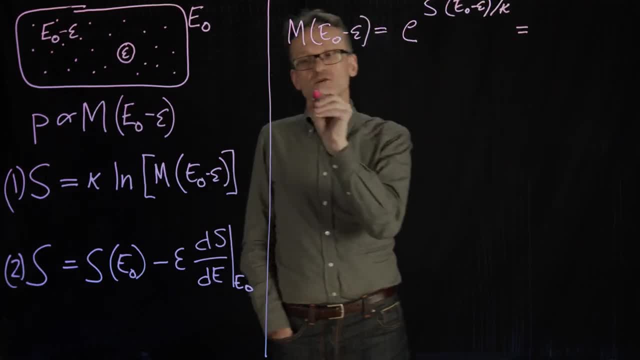 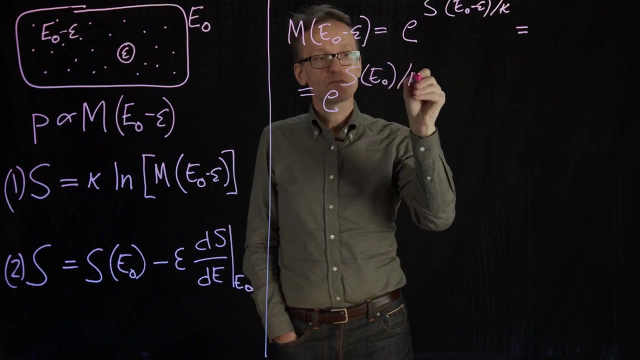 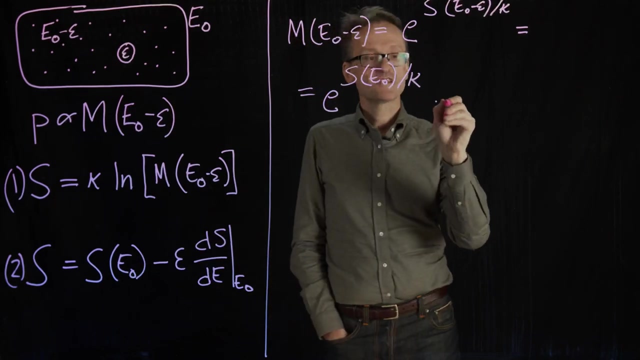 That's just the plain definition. So let's then insert equation 2 here. That corresponds to the exponential, the first term s at the value e0 divided by kappa Minus. well, the addition here corresponds to multiplication right. 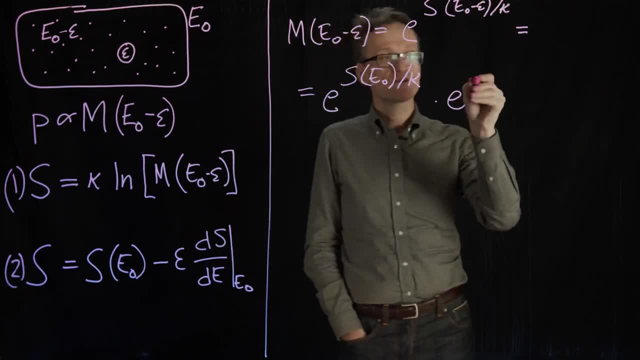 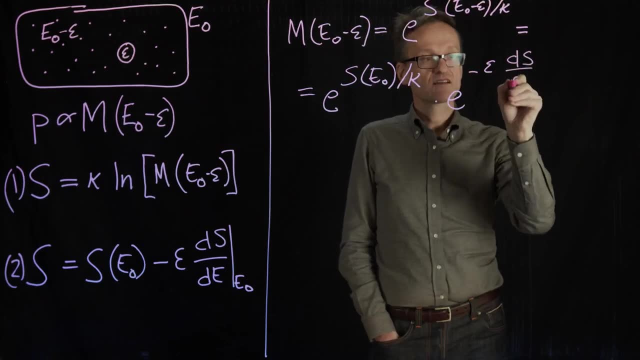 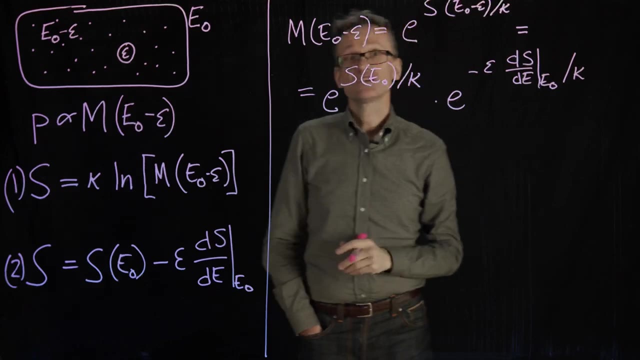 So I can make this a separate exponential and then have a minus sign up here, e raised to minus epsilon, And then I'm going to need that entire expression, ds de taken at the value e0 divided by kappa, And this might not look simple, but you're done. 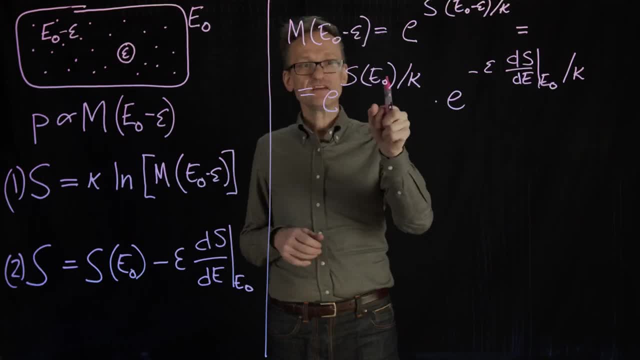 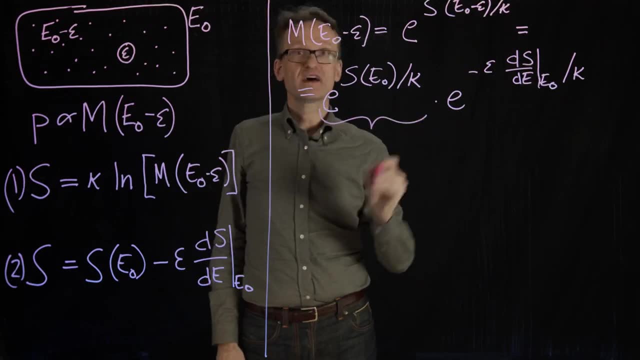 This is amazing s of e0, the whole point here is that e0 is constant when I look at the world, So this is going to be one big fat constant factor, And we're interesting things. we're talking about proportionality. 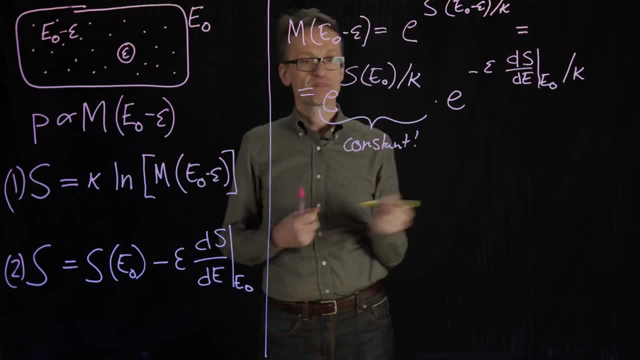 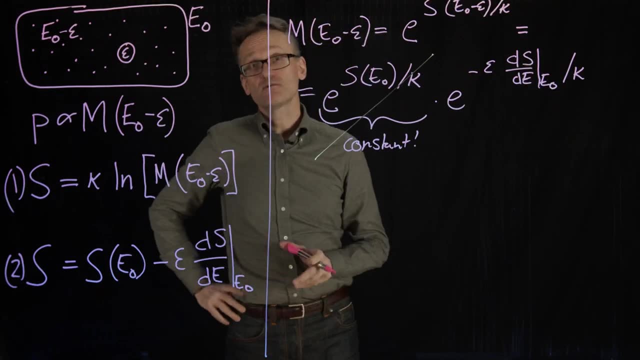 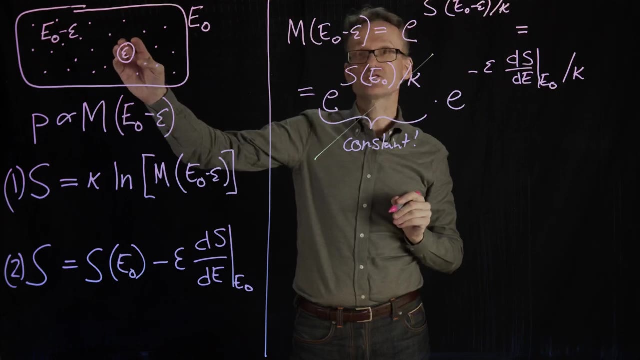 So who cares about the constant? We can strike that out Here. things look more complicated, though. You could argue that if we were defining physics, we might say that the energy here. somehow that depends on how much energy I have in the small system. 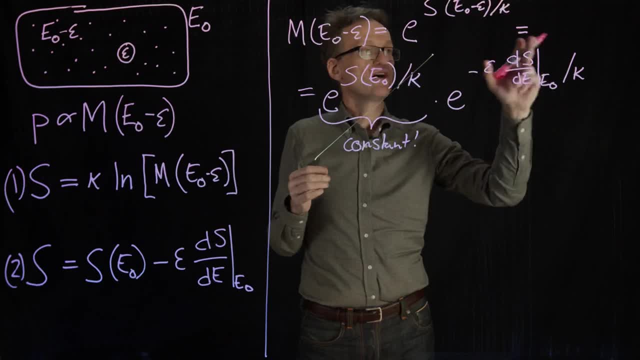 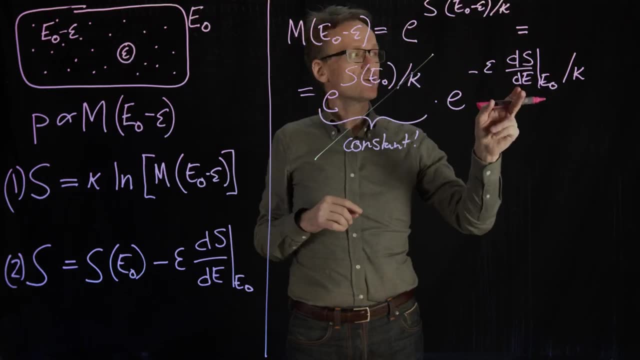 So that's definitely something that I have to consider, While this whole other part has to do with derivatives and connections, how entropy is changing relative to energy. So somehow the second term here describes as I'm exchanging energy. how would that influence the number of states? 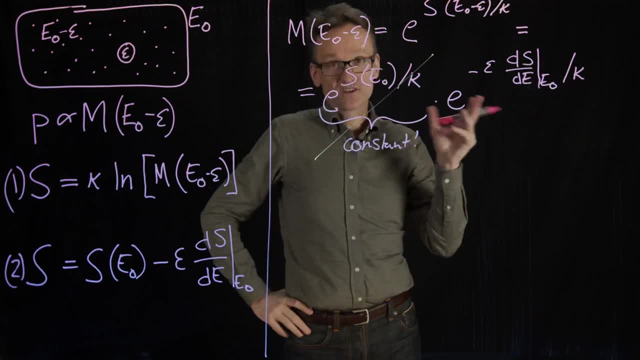 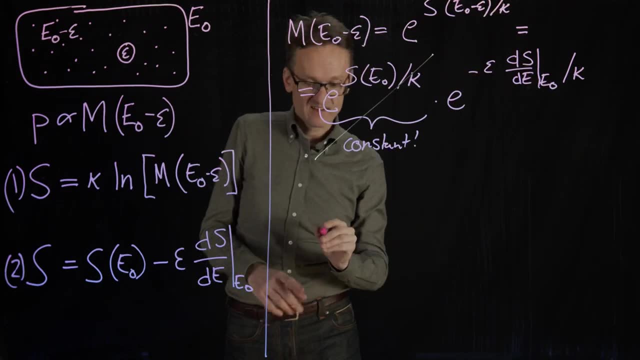 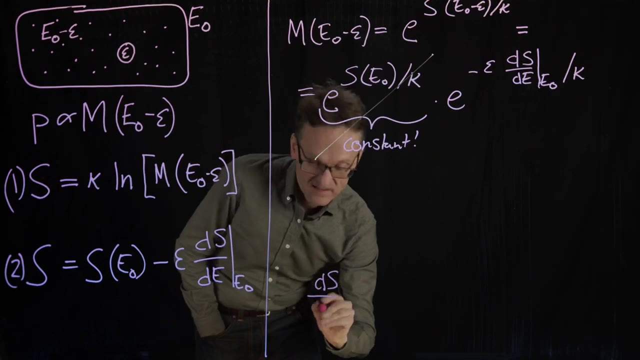 I would likely have called that x if I saw this the first time, But the point is that we're not the first ones to see this, So if you do that math- actually, I'm going to move down here- It turns out that ds de corresponds to 1 over t. 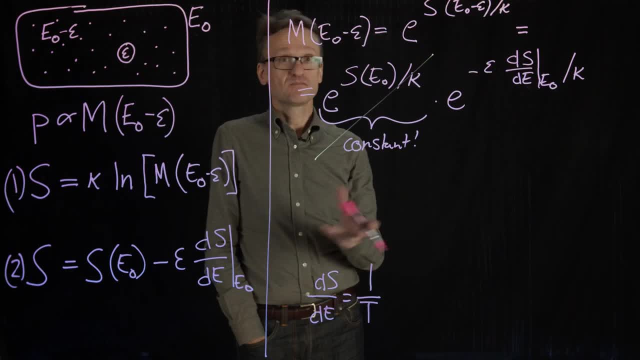 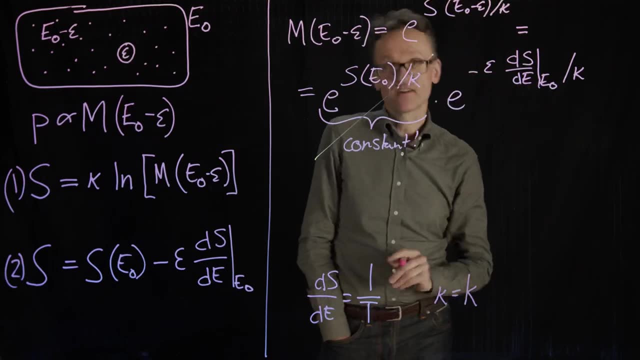 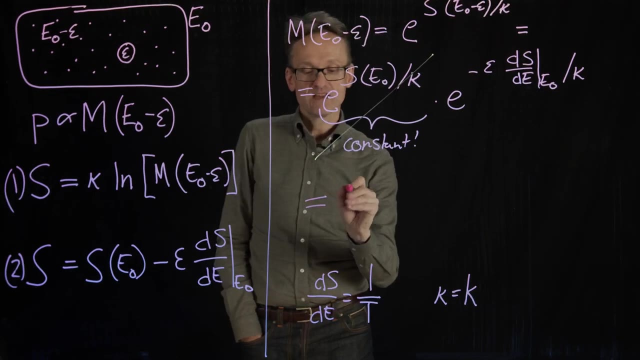 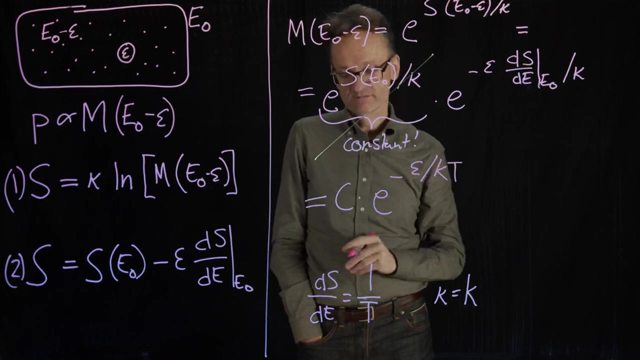 Instead of x I can say 1 over t. It's just a number for now. And instead of kappa let's put k there. Let's call kappa. that seems to be a fundamental constant. That will mean that this m equals a constant times e raised to minus epsilon divided by kt. 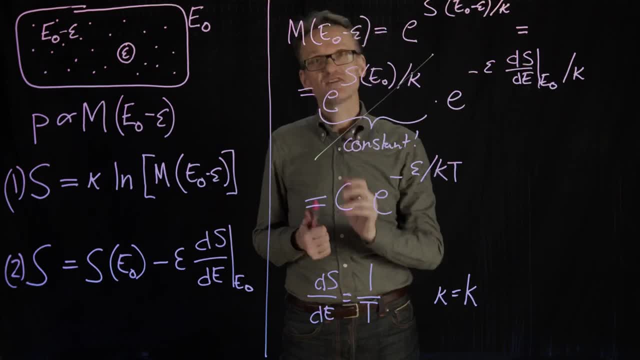 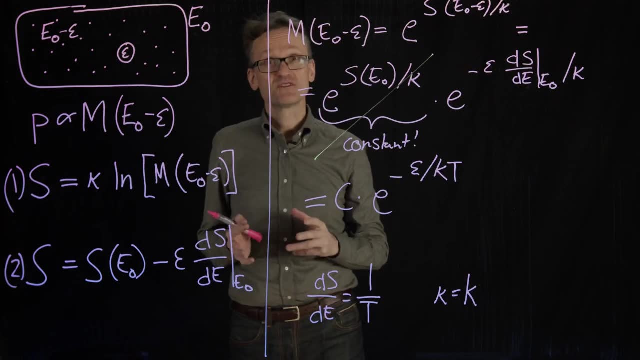 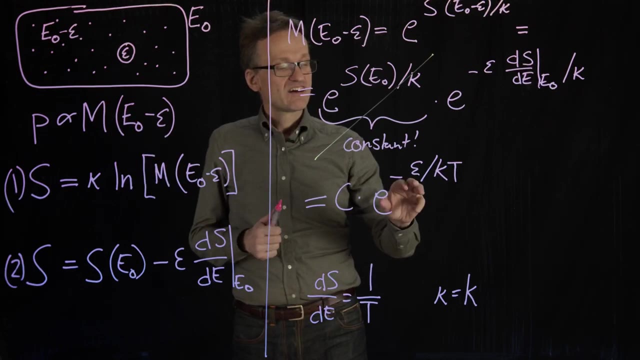 And that is the proportionality you were looking for. right, We have re-derived the Boltzmann distribution. But the cool thing, we have now derived the Boltzmann distribution without really assuming anything. This can be any system, And remember, the entropy came out naturally here.